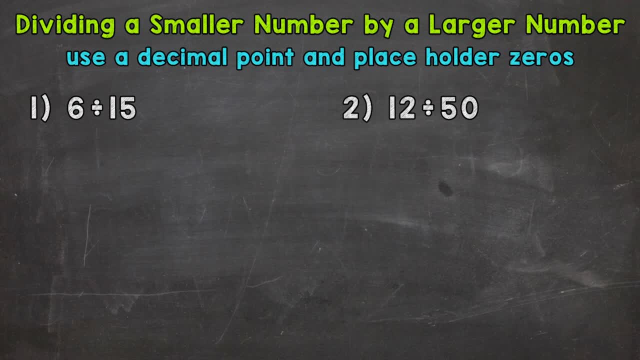 and placeholder zeros in order to go through our division process. So let's jump into number one and see exactly how we solve these types of problems. So for number one, we have 6 divided by 15, and the first thing we want to do is set this problem. 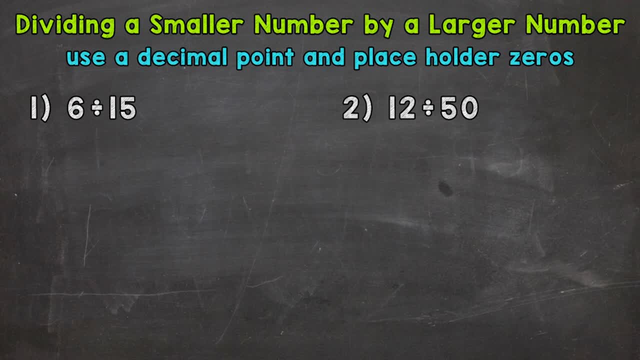 up Now. don't worry about which number is larger in value or smaller in value. That has nothing to do with how we're going to set this division problem up. We need to take a look at the order of the problem and what this problem means. So again, we have 6 divided by 15.. So 6 is being 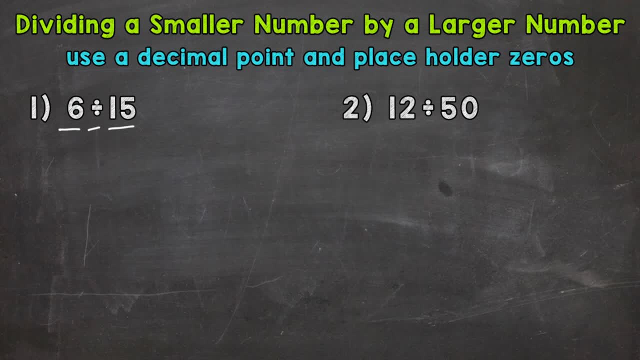 divided or split up. So that's what we call our dividend. It's what goes under our division bar Now, 15 is what we are dividing by. It's what we call the divisor. So it is going to go on the outside. Now that may. 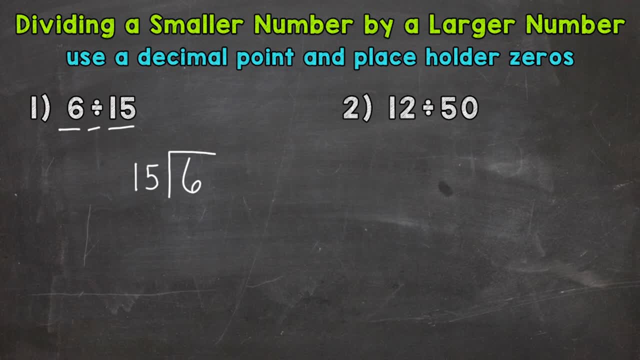 look like it's off or incorrect, but that is correct. We have 6 divided by 15.. Again, don't worry about which number is larger or smaller when we set up division problems. This is not going to happen. We're going to have 6 divided by 15.. We're going to have 15 divided by 6.. These 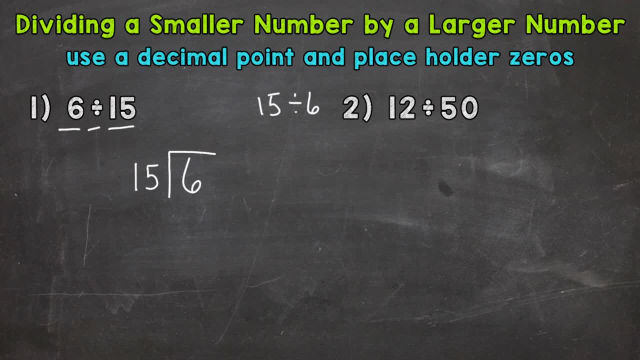 are two different problems: 15 divided by 6, the larger number in value would happen to be under the division bar and the 6 would be on the outside. But again, that's not what we have. We have 6 divided by 15.. So we're starting with 6 wholes and dividing or splitting it into 15 equal. 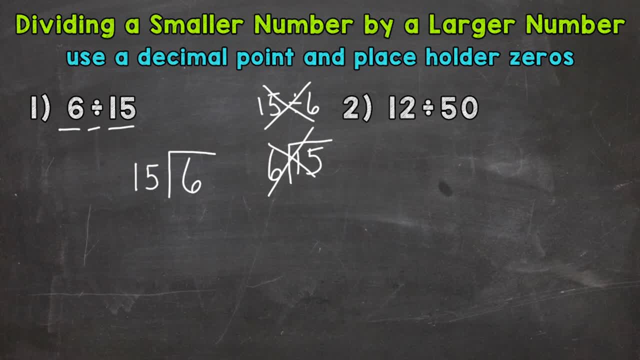 groups. So our answer is actually going to be less than one whole. So let's see how we solve this, And we'll start with our division process. So divide: How many whole groups of 15 can I pull out of 6? Well, I can't do that, So 0.. We cannot pull any whole groups of 15 out of 6.. Multiply: 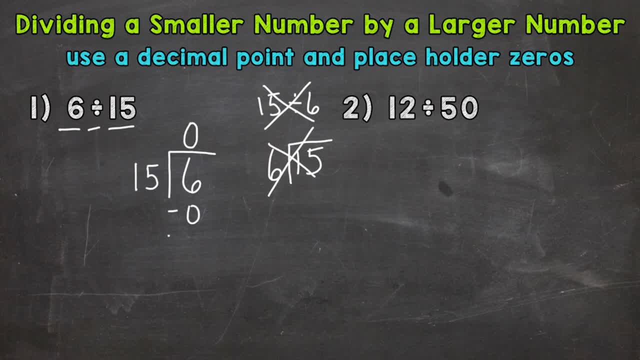 0 times 15 is 0.. Subtract 6 minus 0 is 6.. So in order to continue here, we need to bring something down. So what we're going to do, we're going to place a decimal point after. 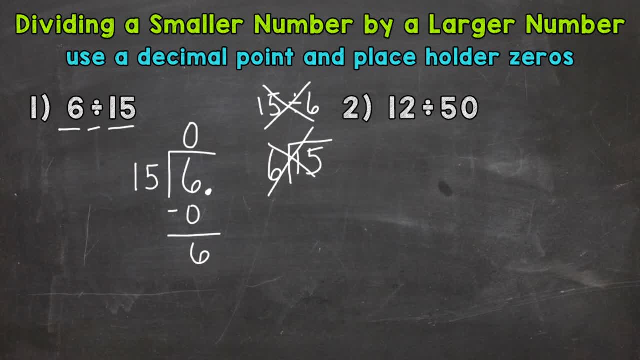 6.. So we can place a decimal point after a whole number. The value of that 6 is still 6.. We didn't change the problem at all. So once you place that decimal point, bring it straight up. That's going. 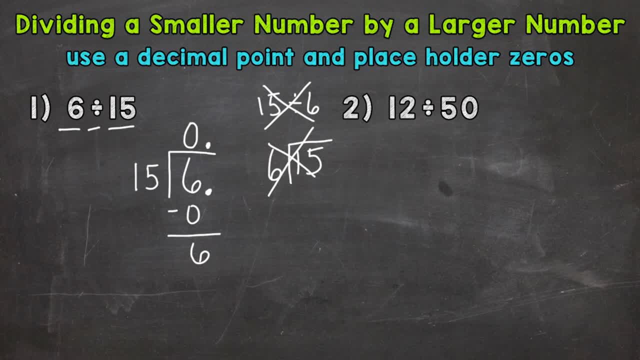 to place it in our answer correctly. So we need something to bring down. So what we can do, we can place a 0 to the right of that decimal. Again, that doesn't change the value of the 6 or the value of the problem. So we can do that. So now 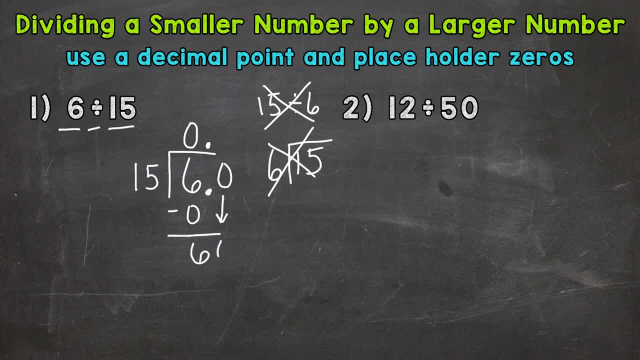 let's bring that 0 down and continue our process. So now we have 60 divided by 15.. How many whole groups of 15 out of 60?? Well, 4.. That hits 60 exactly. So 4 times 15 is 60.. 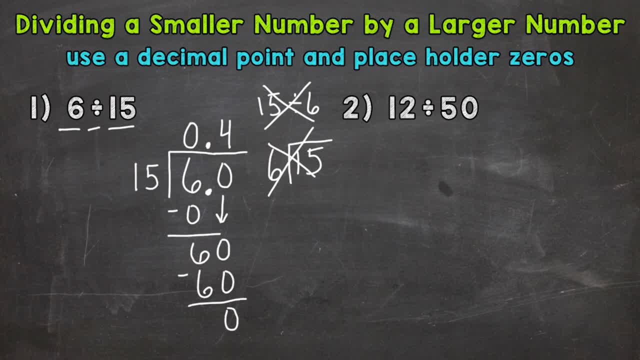 Subtract And we get 0.. So we are done. Our answer is 4 tenths. Again, we got an answer less than one whole. Think about it: We got an answer less than one whole. So we got an answer less than. 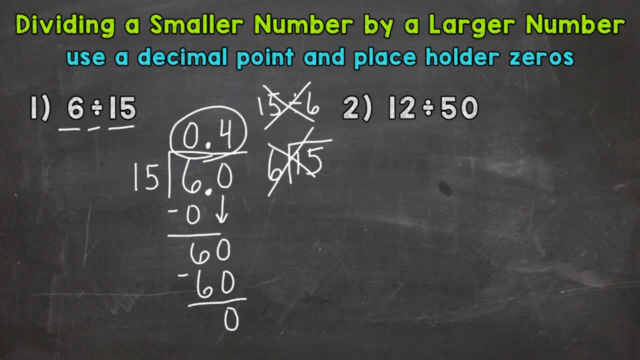 We split those 6 wholes into 15 equal groups, So we didn't have enough for one whole in each of those groups, So we ended up with 4 tenths as our answer, or the value of each of those 15 groups. So let's move on to number 2, where we have 12 divided by 50. Again, don't worry about which. 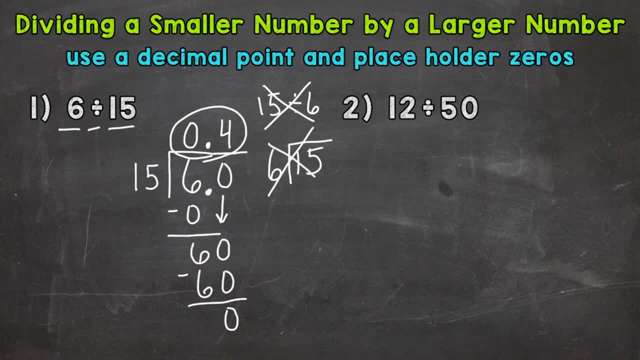 number is smaller or larger in value. Worry about the order and what that problem means. So we have 12 divided by 50. So 12 is our dividend. It's what's being divided or split up. So that goes under our division bar. 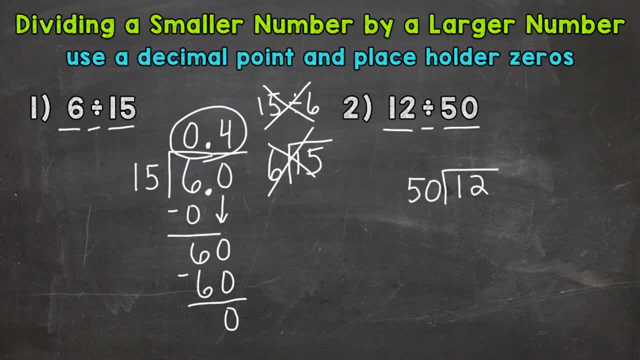 and the 50 goes on the outside. Now we're all set up and ready to go through our division process. So how many whole groups of 50 out of 1?? Well, we can't do that. So how many whole groups of 50 out? 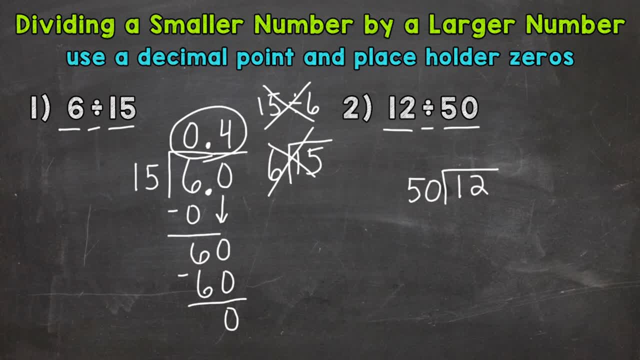 of 12?? Well, we can't do that either. We can't pull a whole group of 50 out of 12.. So let's put a 0 there To hold this place. 0 times 50 is 0. Subtract, we get 12.. So now we're stuck. So what we can do: 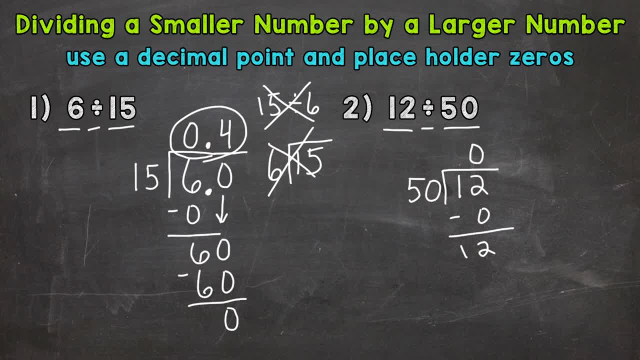 we can use a decimal point and placeholder zeros. So let's put our decimal point after 12.. Again, that does not change the value of our problem, or that 12.. Bring that decimal point straight up and that will place it correctly in our answer. So we need something to bring down. So what we can do. 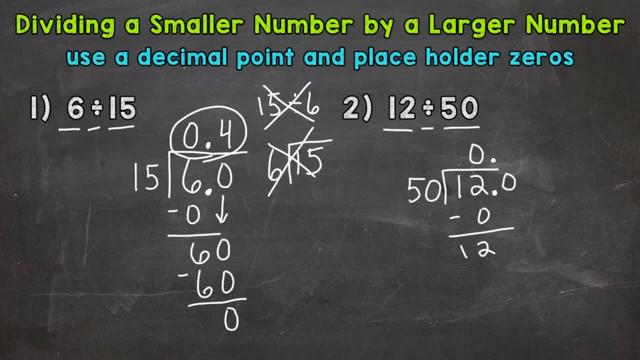 we can use a placeholder zero in the 10th place. Again, doesn't change the value of anything and bring that zero down. So how many whole groups of 50 out of 120?? Well, 2. That gets us to 100 and 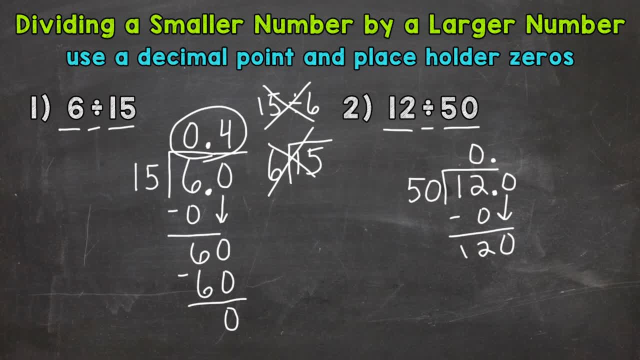 that's as close as we can get to 120.. So 2. Let me extend this division. bar there 2 times 50 is 100.. Subtract and we get 20.. So we are still not done. So what we can do, we can use another placeholder, zero. Let's place one. 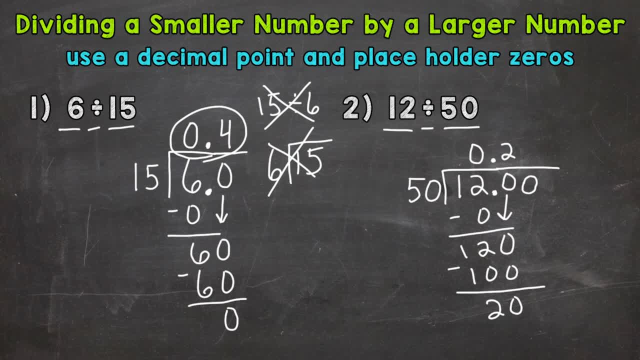 in the 100th place, Again not changing the value of anything, and we can bring that down. So now we have 200 divided by 50. How many whole groups of 50 out of 200? 4. That hits 200 exactly. So this is. 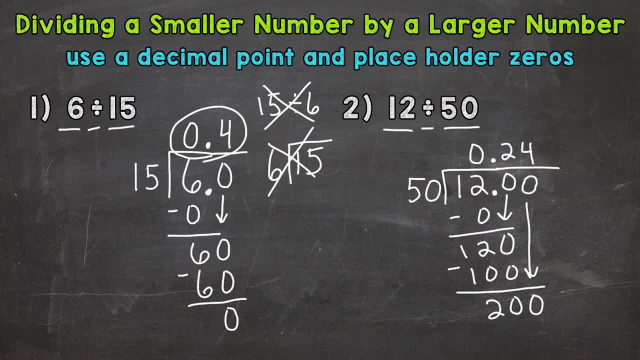 going to be our last digit in our answer, But let's wrap everything up with our process. So now we need to multiply: 4 times 50 is 100.. So now we have 200.. So now we need to multiply 4 times 50 is. 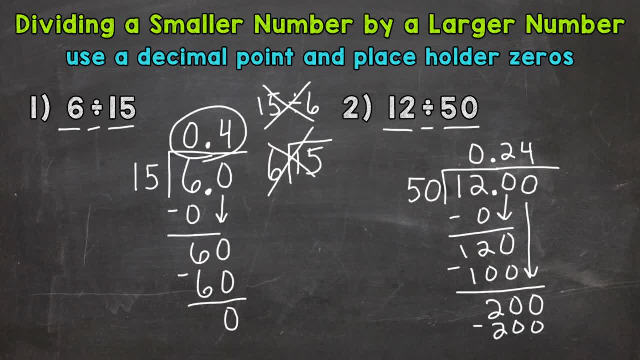 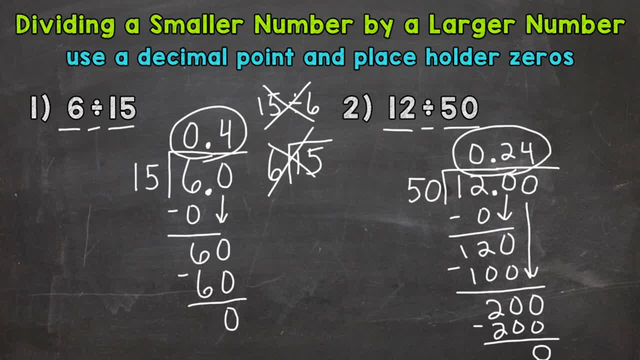 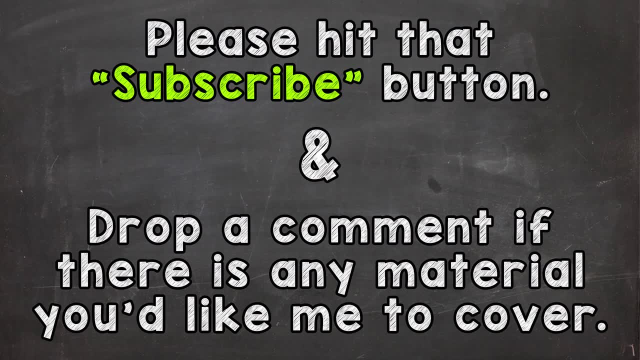